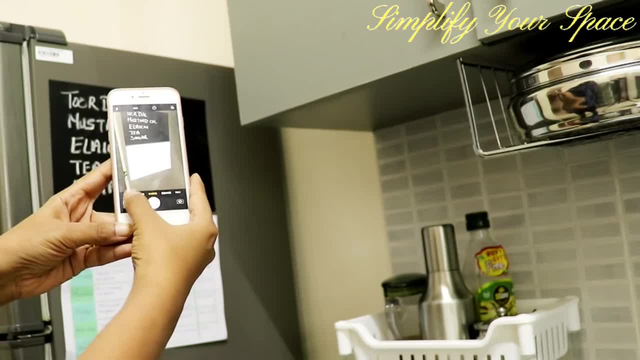 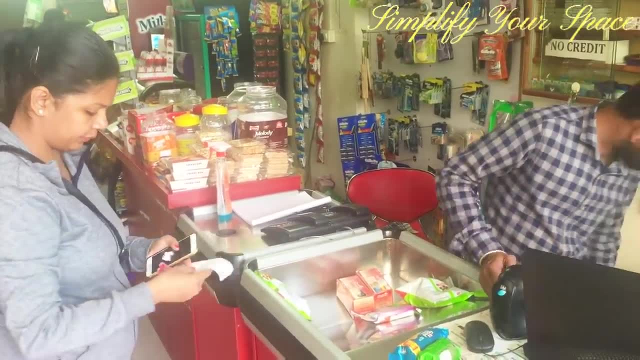 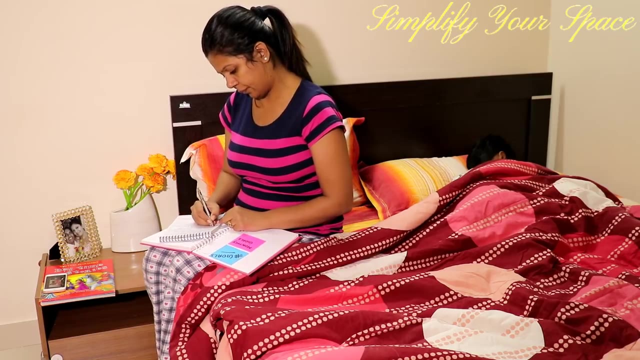 finish. Click a picture while going for the grocery shopping so that you don't forget to buy anything which will save you from another trip to the grocery store. Use your daily planner to write down your to-do list, appointments and goals for the next day so that you don't forget. 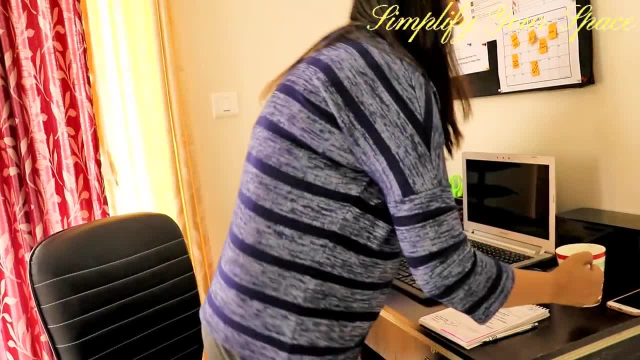 anything important. When you finish your daily schedule, you can start planning your day. If you don't have a planner, you don't have to worry about it. Check the planner as soon as you wake up and plan your day according to the list. Jotting everything down makes sure you complete all. 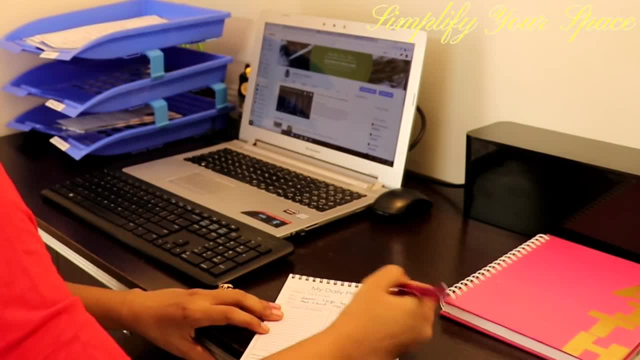 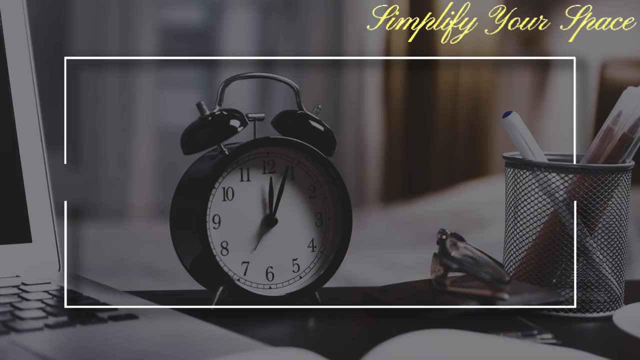 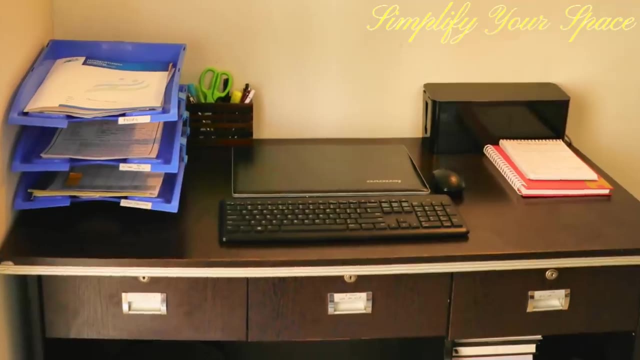 the tasks before the day ends. Also, write down your major goals on the top of the page to stay motivated while working. It will boost up your energy level whenever you feel low. Keep your working desk clean and organized all the time. Keep your important task list. 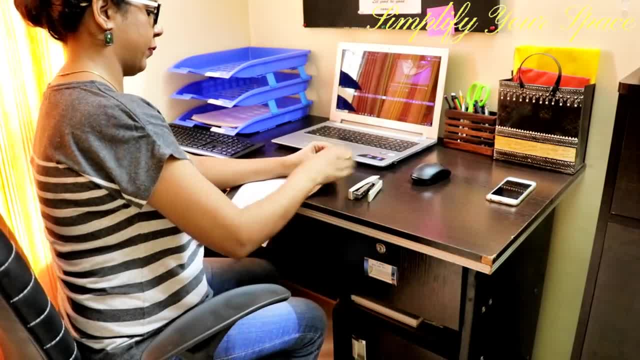 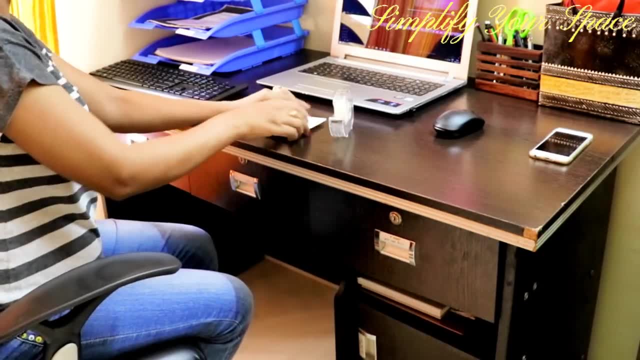 papers and stationery near to your desk. Keep your important task list papers and stationery near to your desk. It is quite irritating to get up and find a paper or scissor while working, which also waste lot of your time. Also, do not clutter up your desk, as that affects your productivity and 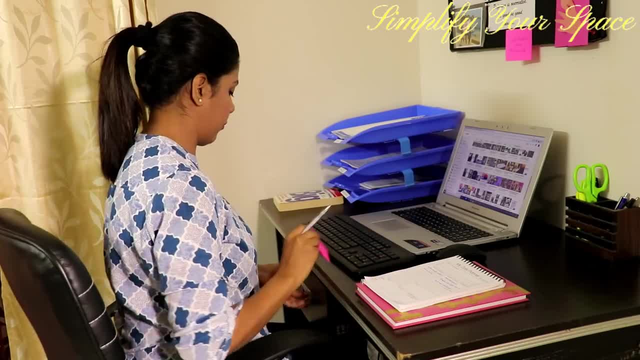 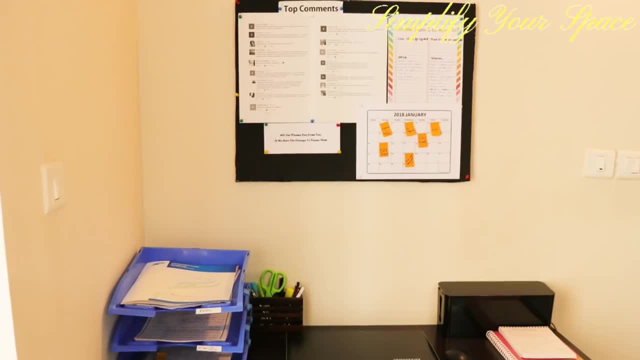 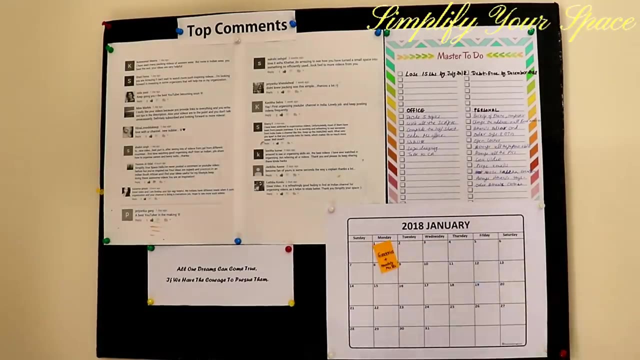 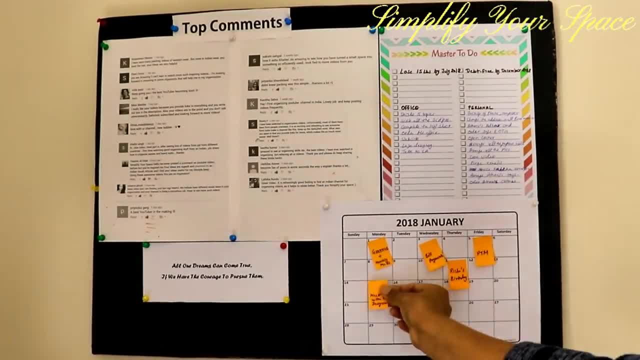 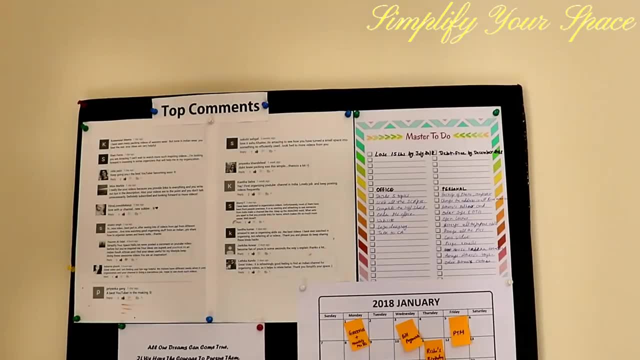 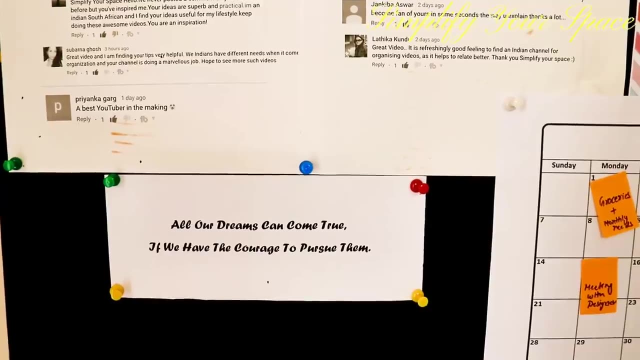 Like bill payments, ptm meetings, grocery shopping, birthdays and anniversaries, etc. Plan your day accordingly, which will avoid unnecessary havoc and late payments. Pin or write your goals, tasks and important notes. Also write a motivational quote or paste a vision board to keep you motivated all the time, Like I have this board just above my working desk. 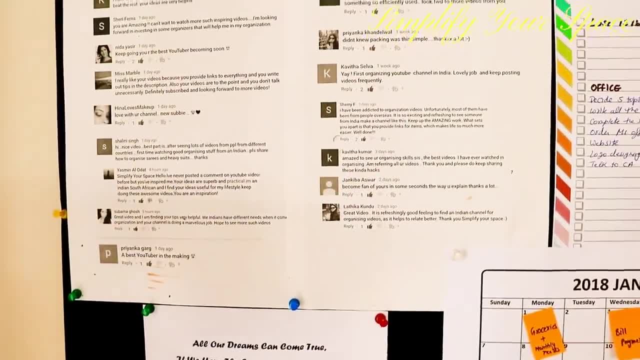 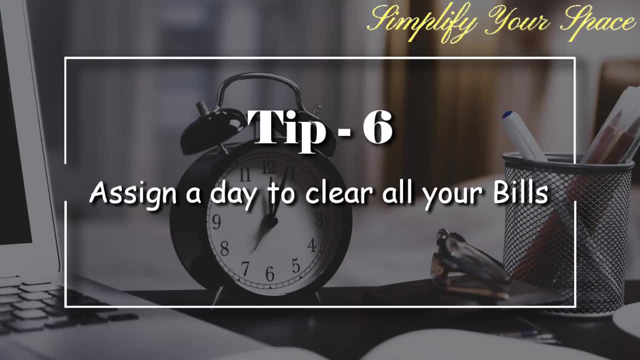 I have taken the print out of your lovely comments and pasted here. It really keeps me motivated all the time and brings a smile on my face whenever I see it. Assign a day to pay all your bills- house rent and grocery. Do not waste time every day to pay bills. 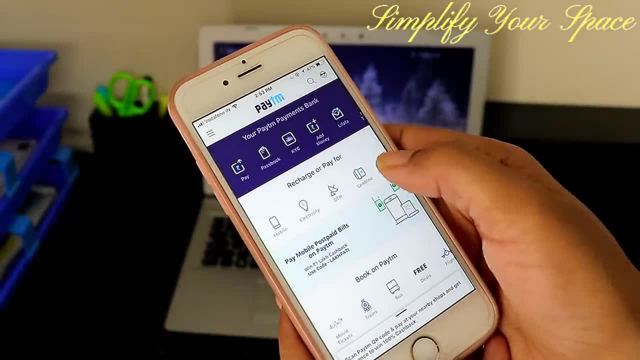 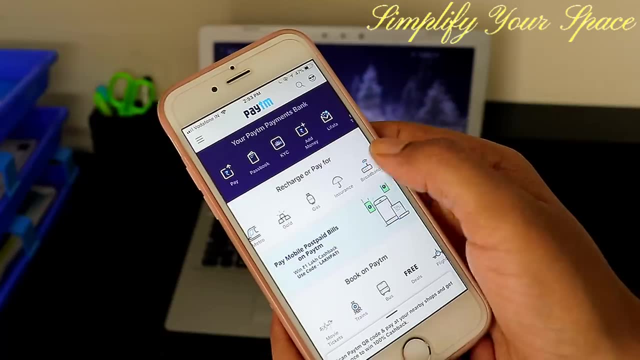 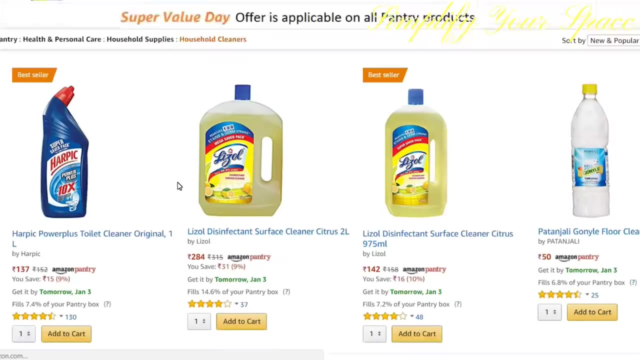 Best is to use bill payment apps like ptm or free charge and pay all your bills instantly while sitting in the comfort of your home. like phone, gas, electricity, cable water, internet, school and institute. You can also order your groceries and monthly needs online. Every month, from 1st to 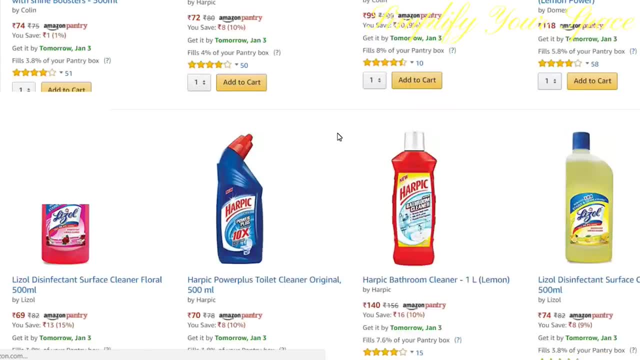 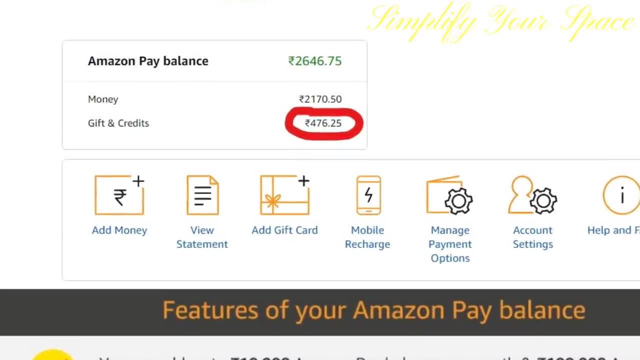 12th of every month, the bill payment app will be available on your phone. You can also use bill payment apps like paypal, google play and amazon app. All these apps will offer big saving days. You get all the groceries and household items on the. 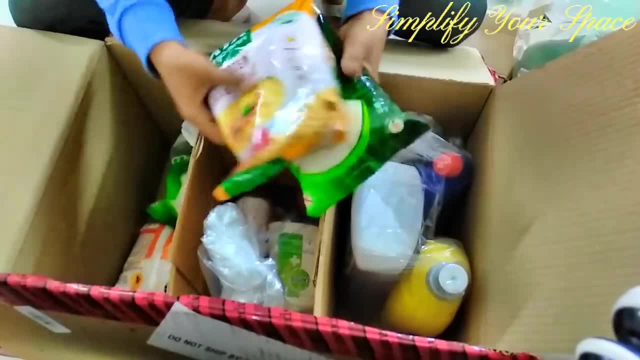 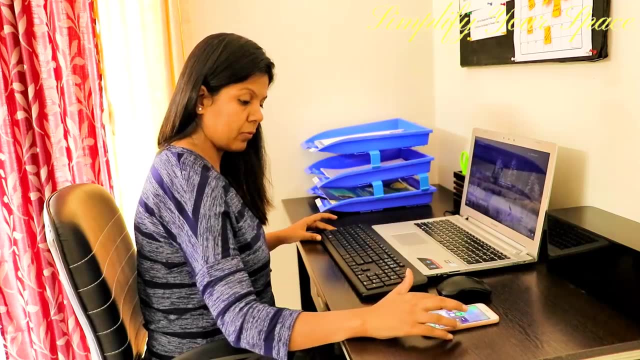 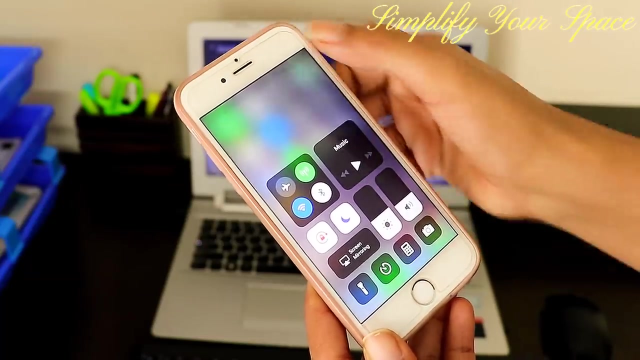 discounted prices as well as lot of cash back. Best thing is: amazon delivers these items next day itself if you are a prime member. Stay out from all the distractions while working or doing something important: whatsapp and social media on your phone. how many times it happened that while working, you picked? 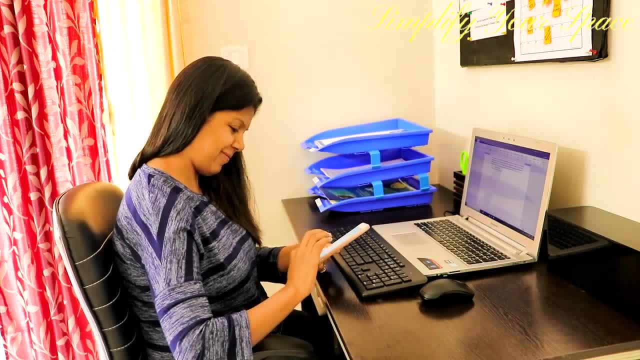 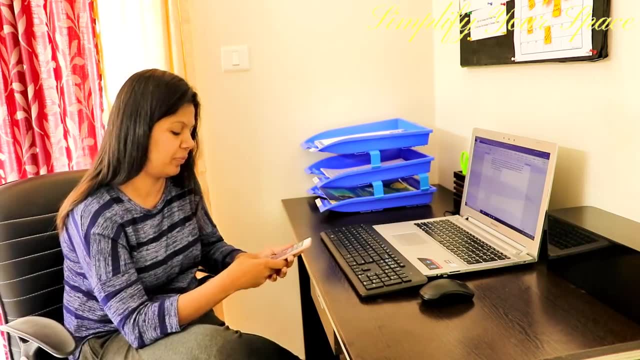 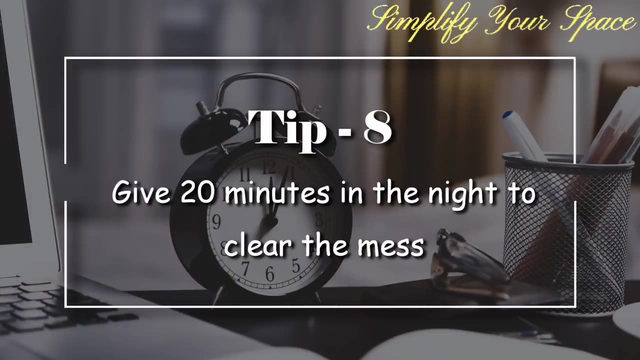 up your phone to read one message and ended up spending an hour on chatting, browsing or checking social media. i'm not asking you to stop it forever, but assign the time to see your phone or to check social media. give 15-20 minutes in the night to organize the clutter and keep things in the 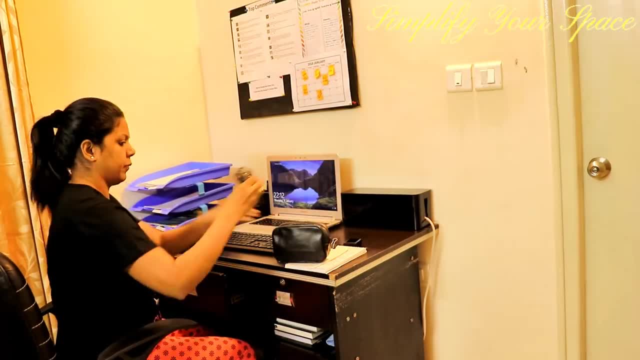 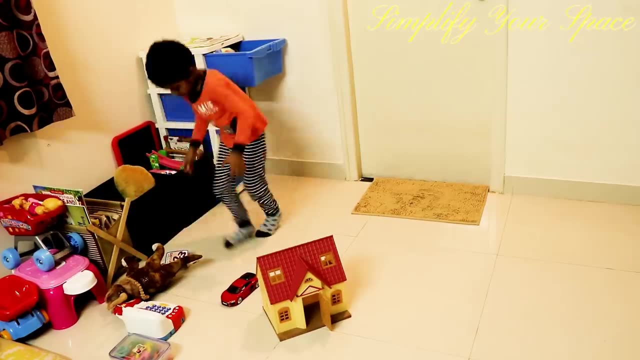 designated place. clean the kitchen counter, remove the mess from your desk and pick up the toys from the floor. take a help of your kids. let them develop this habit to stay organized and clear the clutter after playing. this will save your time in the morning and will make you more efficient. 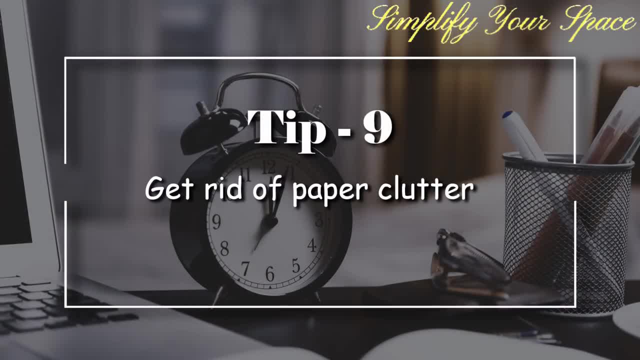 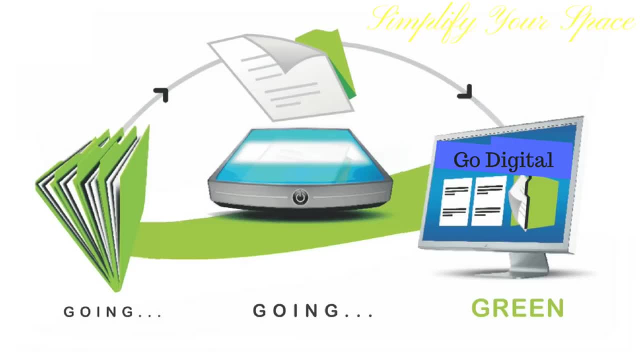 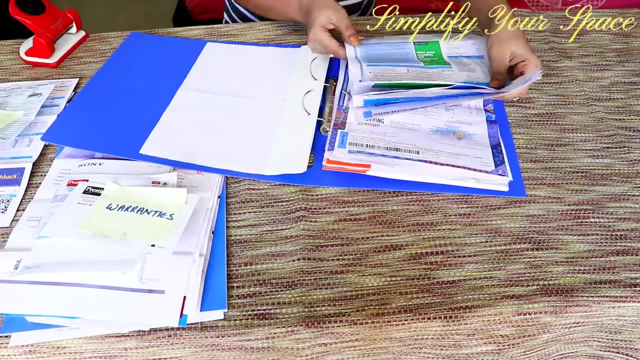 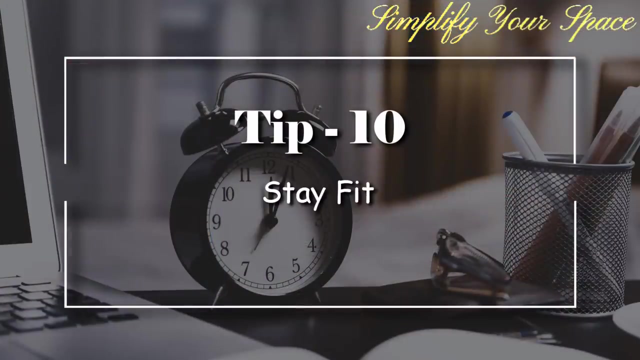 and productive. file your important papers every month before you transform into a tower. go green and stop accepting paper bills. request to get digital bills via email which can be stored in various storage devices, both online and offline. this will save your time to file them every month. all these points are meaningless and waste if you don't eat proper food, exercise, stay healthy and 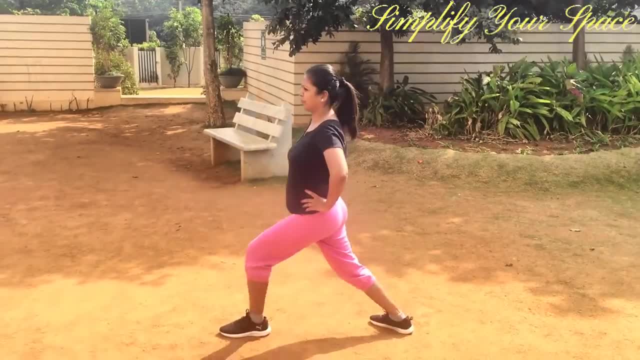 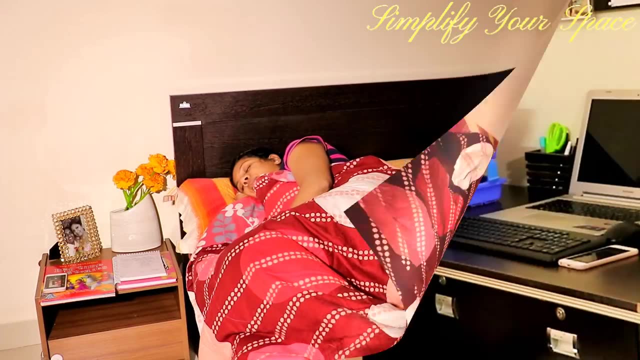 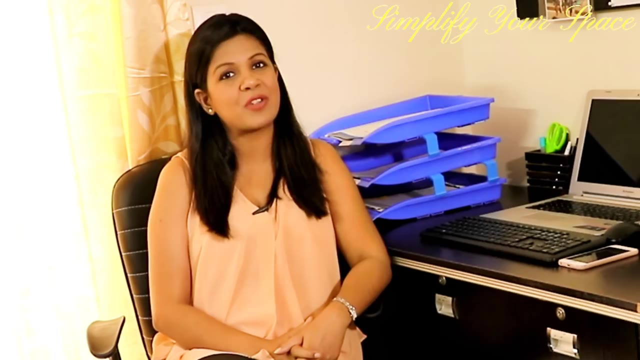 sleep well for every day at least eight to nine hours proper sleep, exercise and eating healthily boost energy levels, clear your mind and allow you to focus. clearly also staying happy is very important. happier people are way more productive. if you have missed with this article on how to stay happy, then the link.